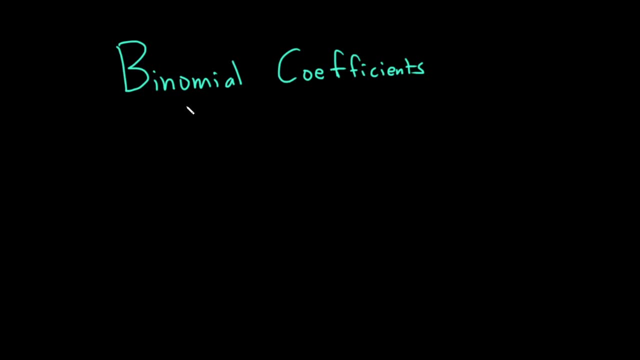 Hi, in this problem we're going to do some examples of computing binomial coefficients. So the formula that we're going to be using is n choose r, and this is equal to n factorial all divided by n minus r factorial times r factorial. So this tells you the number of ways to choose r objects from a group of n objects. 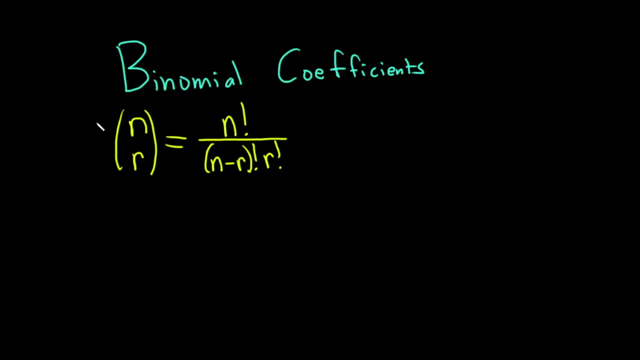 Okay, let's do some examples with various numbers. Let's start with 7, choose 4.. So, just applying the formula, we have n equals 7 and r is 4, so this is 7 factorial over, and then it'll be n equals 4.. 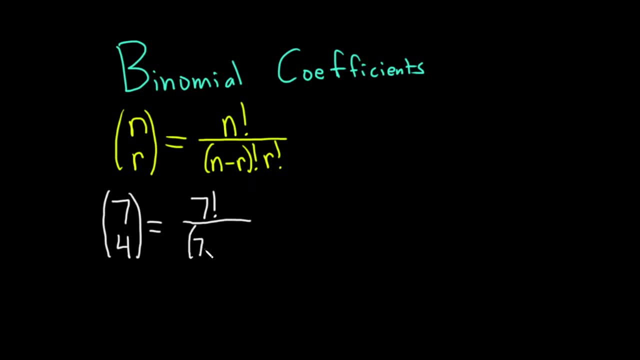 So we have n minus r, so it'll be 7 minus 4 factorial. and then r. well, r is just 4, so this is 4 factorial. This is equal to 7 factorial over 7 minus 4, that's going to be 3 factorial. 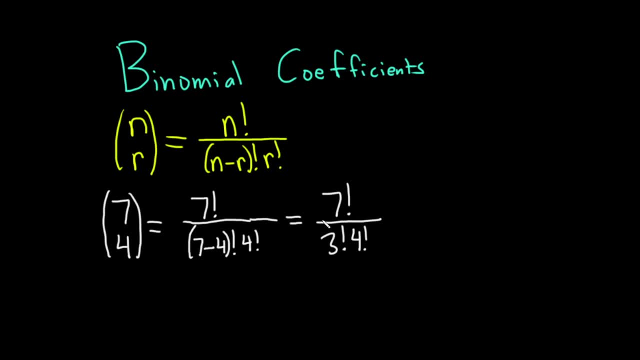 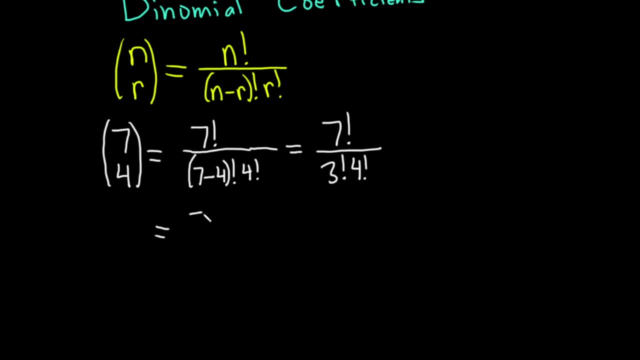 Then here we have 4 factorial still. So there's a couple ways to do this. Here's one way. So 7 factorial is really 7 times, 6 times, 5 times, and then it's 4,, 3,, 2, 1, which is 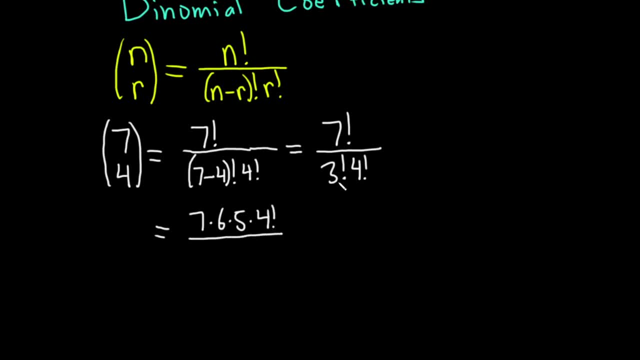 the same thing as 4 factorial over 3 factorial is 6, and then we have 4 factorial These. cancel these. cancel 7 times 5 is 35. Boom, There it is. Let's do another one, just so you get more practice. 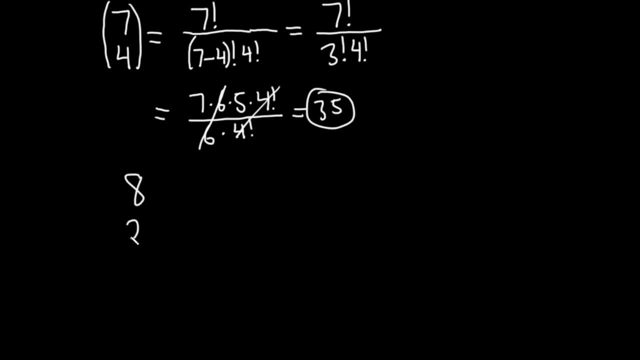 I'll do this next example a little bit differently. Let's do 8 choose 2.. So this will be 8 factorial over, that's the n factorial over n minus r, So 8 minus 2 factorial, And then again r factorial, so 2 factorial. 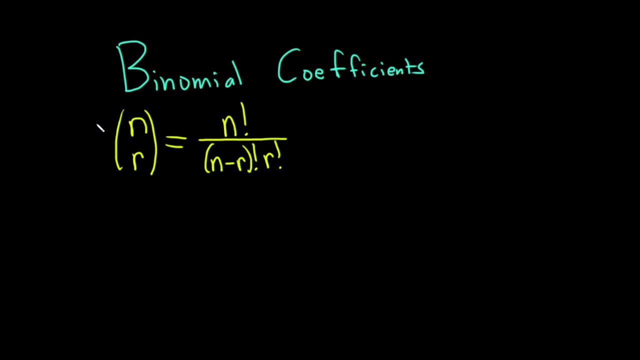 Okay, let's do some examples with various numbers. Let's start with 7, choose 4.. So, just applying the formula, we have n equals 7 and r is 4, so this is 7 factorial over, and then it'll be n equals 4.. 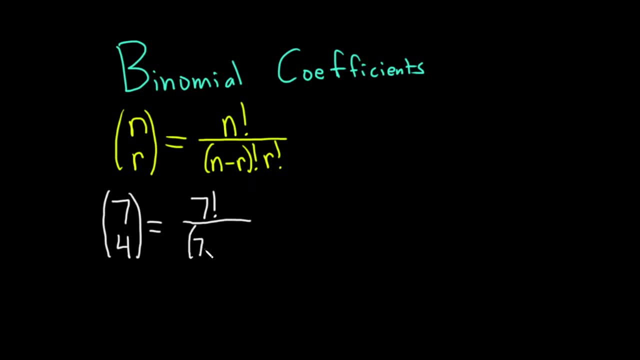 So we have n minus r, so it'll be 7 minus 4 factorial. and then r. well, r is just 4, so this is 4 factorial. This is equal to 7 factorial over 7 minus 4, that's going to be 3 factorial. 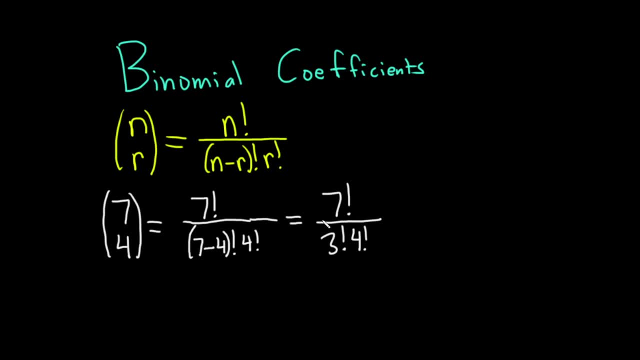 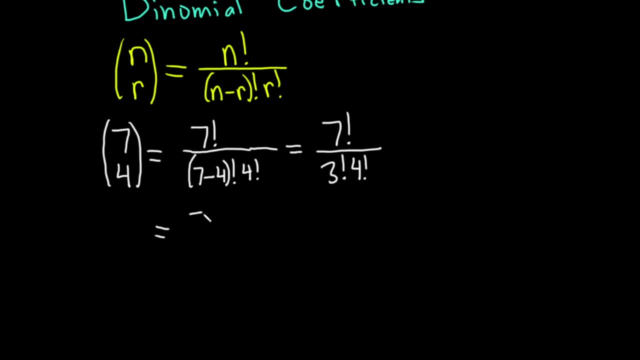 Then here we have 4 factorial still. So there's a couple ways to do this. Here's one way. So 7 factorial is really 7 times, 6 times, 5 times, and then it's 4,, 3,, 2, 1, which is 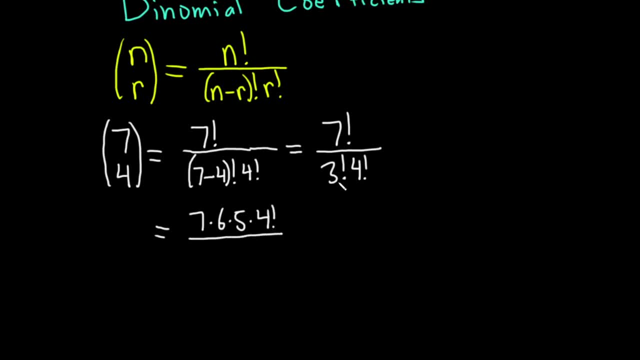 the same thing as 4 factorial over 3 factorial is 6, and then we have 4 factorial These. cancel these. cancel 7 times 5 is 35. Boom, There it is. Let's do another one, just so you get more practice. 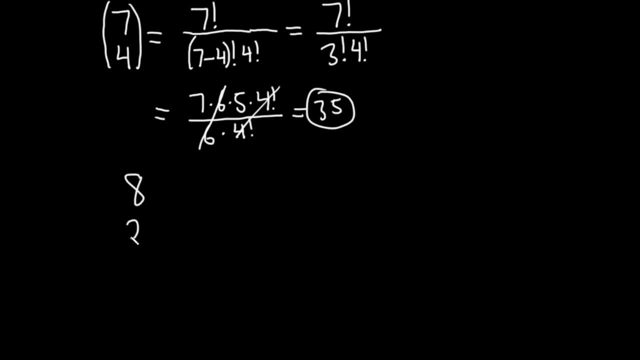 I'll do this next example a little bit differently. Let's do 8 choose 2.. So this will be 8 factorial over, that's the n factorial over n minus r, So 8 minus 2 factorial, And then again r factorial, so 2 factorial. 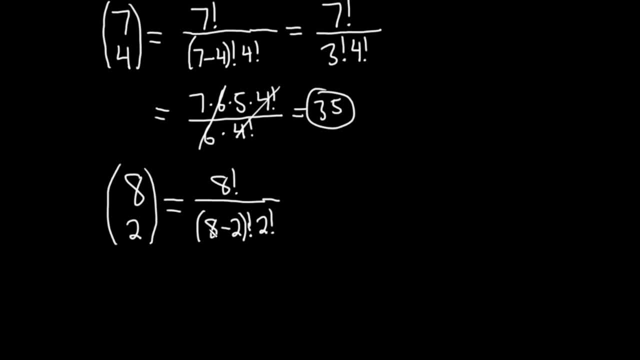 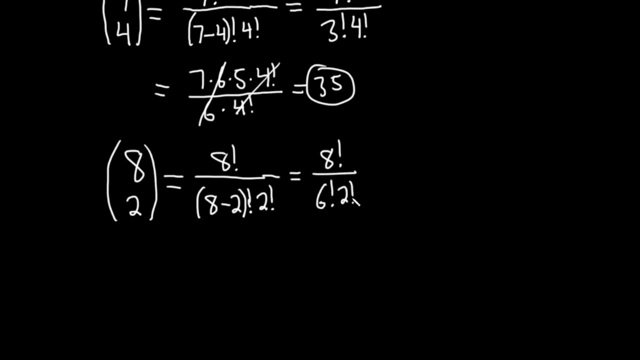 So it's n factorial over n minus r. So 8 minus 2 factorial. It's n factorial over n minus r. factorial, r factorial. This is equal to 8 factorial over 8 minus 2 is 6.. This is 6 factorial, 2 factorial. 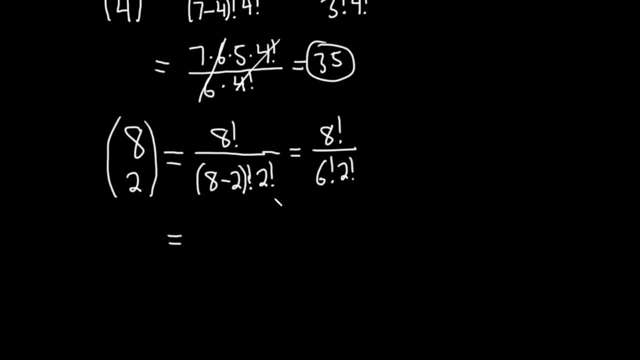 And I said I would do it differently, but I guess I will So you can write it out. You can always. just I took shortcuts here. So 8 factorial is 8 times 7 times 6, 5,, 4,, 3,, 2, 1,, which is 6 factorial. 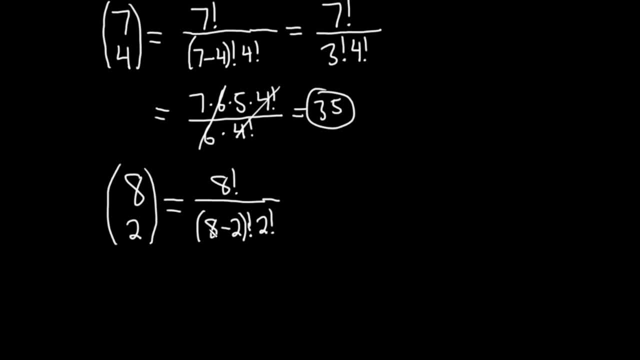 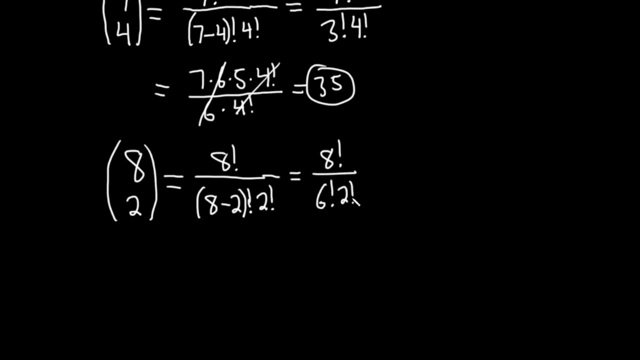 So it's n factorial over n minus r. Let's do 8, choose 2.. It's n factorial over n minus r. factorial, r- factorial. This is equal to 8. factorial over 8 minus 2 is 6.. This is 6 factorial, 2 factorial. 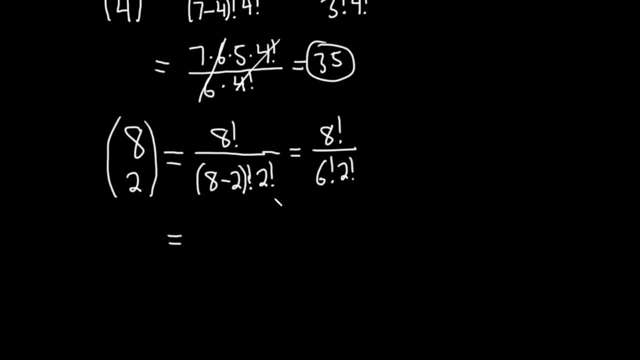 And I said I would do it differently, but I guess I will So you can write it out. You can always. just I took shortcuts here. So 8 factorial is 8 times 7 times 6, 5,, 4,, 3,, 2, 1,, which is 6 factorial. 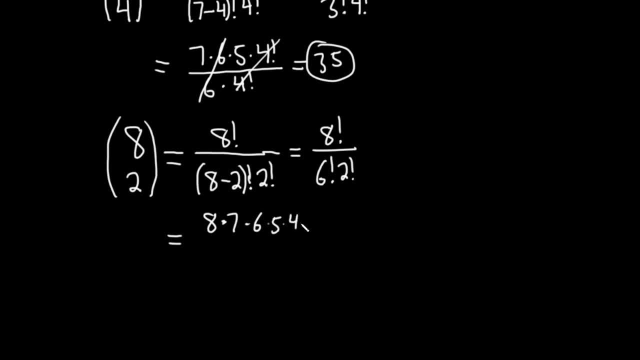 But I'll write it: 6, 5,, 4, 3,, 2,, 1.. And then 6 factorial is 6, 5,, 4,, 3,, 2, 1.. And then 2 factorial is 2 times 1,, so it's 2.. 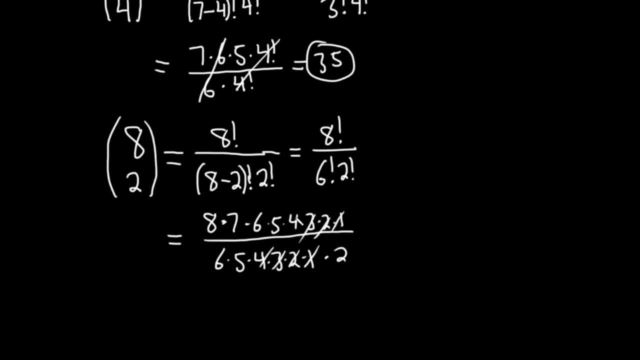 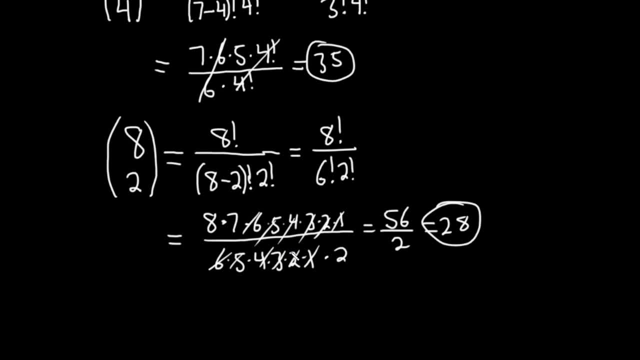 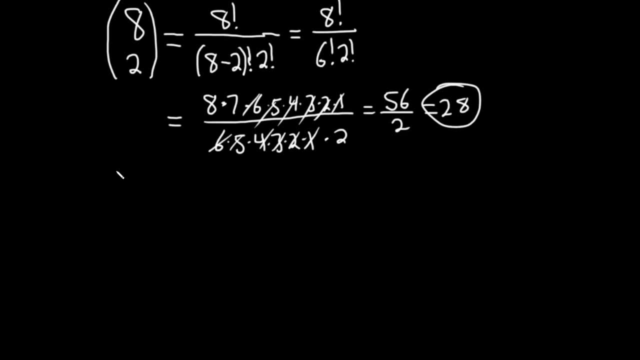 You can always do it that way, It's just, it just takes longer. so I usually don't do it that way. Let's do a couple more examples. How about something a little different? How about something with a 0?? We haven't done that. 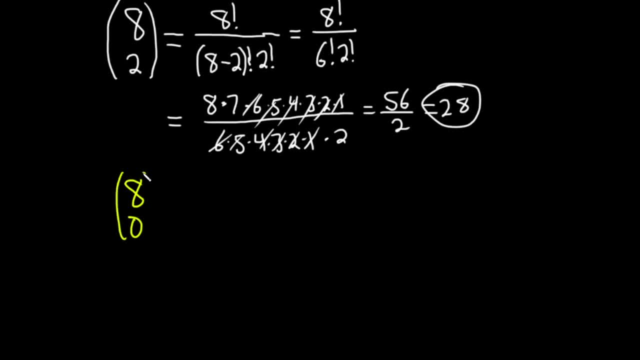 Let's do 8 choose 0, 0, 8 choose 0.. So again the formula is n factorial over n minus r times r factorial, So it's 8 factorial, Then it's n minus r, so 8 minus 0 factorial. 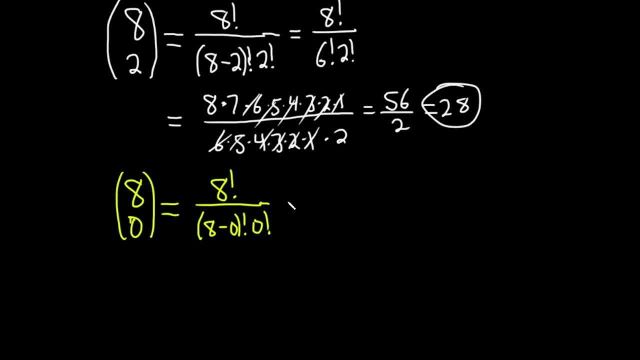 This is equal to 8 factorial over 8 factorial. 0 factorial is 1, boom, you just get 1.. So pretty cool. Notice that you can replace 8 with any number and you're going to get 1.. So, in general, n choose, 0 is going to be 1.. 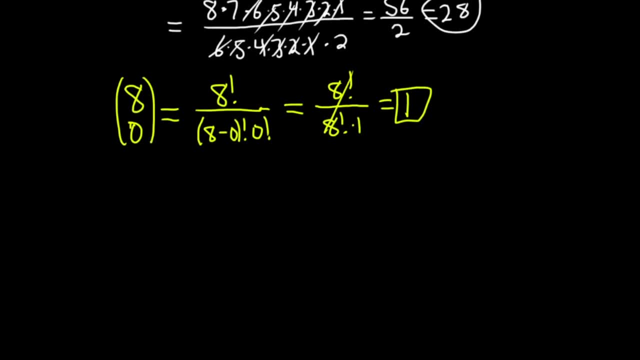 Let's do another one. How about? how about? 7 choose 7,, 7 choose 7.. By the way, this says: how many ways can you choose 0 objects from a group of 8?? There's one way you choose 0 objects. 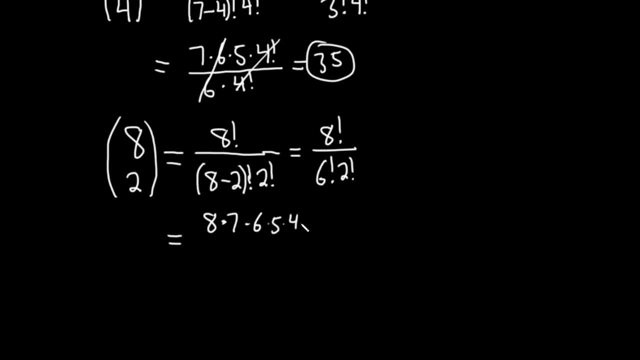 But I'll write it: 6, 5,, 4, 3,, 2,, 1.. And then 6 factorial is 6, 5,, 4,, 3,, 2, 1.. And then 2 factorial is 2 times 1,, so it's 2.. 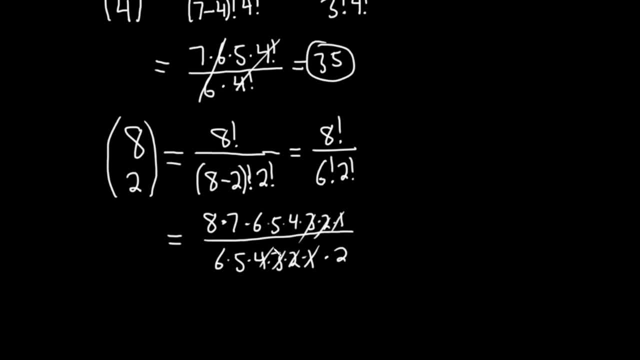 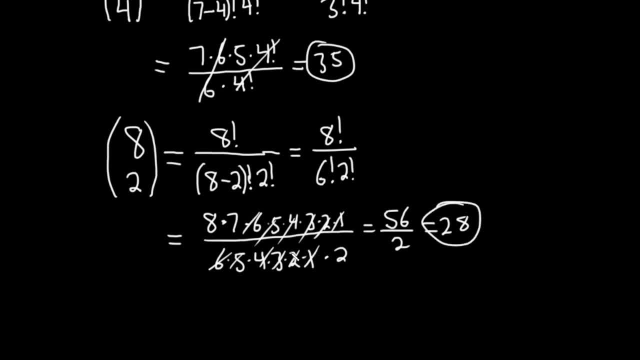 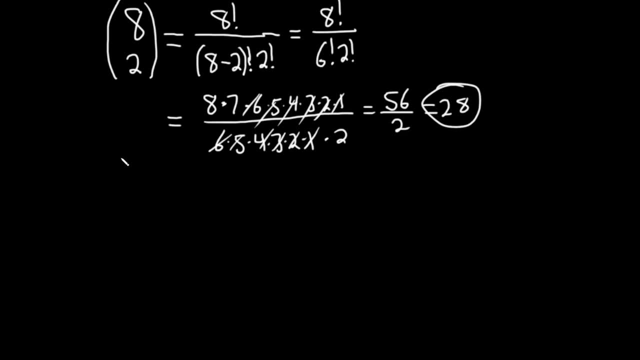 You can always do it that way, It's just, it just takes longer. So I usually don't do it that way. Let's do a couple more examples. How about something a little different? How about something with a 0?? We haven't done that. 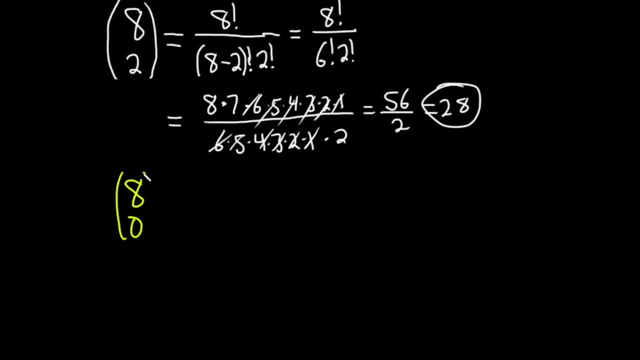 Let's do 8 choose 0, 0, 8 choose 0.. So again the formula is n factorial over n minus r times r factorial, So it's 8 factorial, Then it's n minus r, so 8 minus 0 factorial. 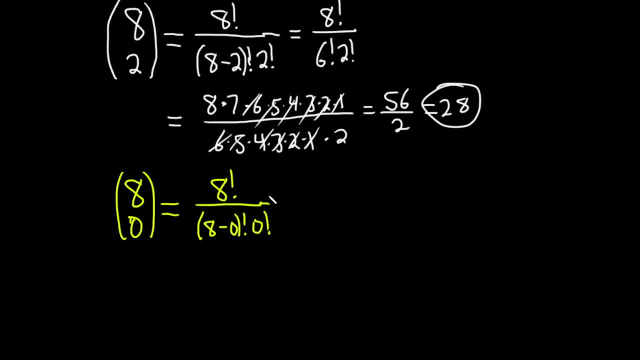 0 factorial. 0 factorial. This is equal to 8 factorial over 8 factorial, 0 factorial is 1.. Boom, You just get 1.. So pretty cool. Notice that you can replace 8 with any number and you're going to get 1.. 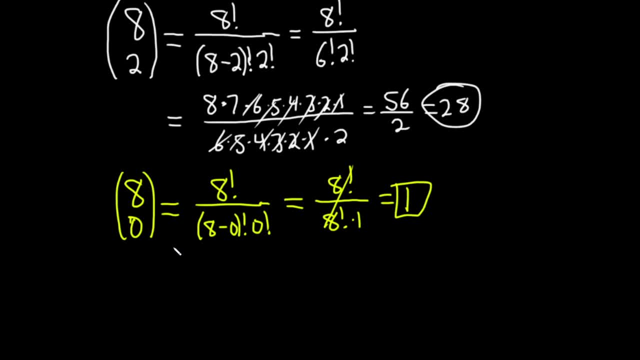 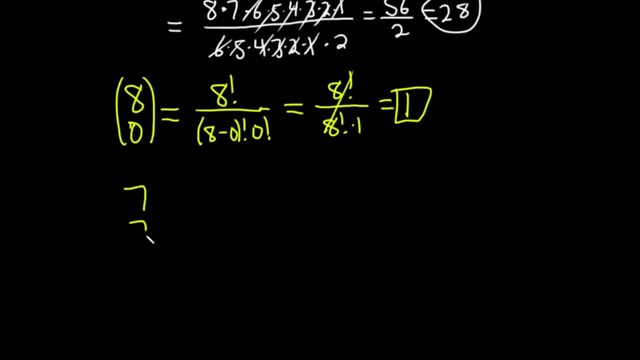 So, in general, n choose 0 is going to be 1.. Let's do another one. Let's do another one. How about 7 choose 7? 7 choose 7.. By the way, this says: how many ways can you choose 0 objects from a group of 8?? 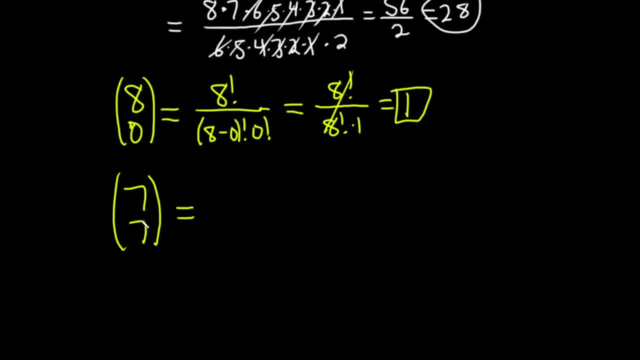 There's one way You choose 0 objects. This one is saying: how many ways can you choose 7 objects from a group of 7?? There's one way: you choose all 7.. So the answer should be 1.. So it's 7 factorial over it's n minus r. 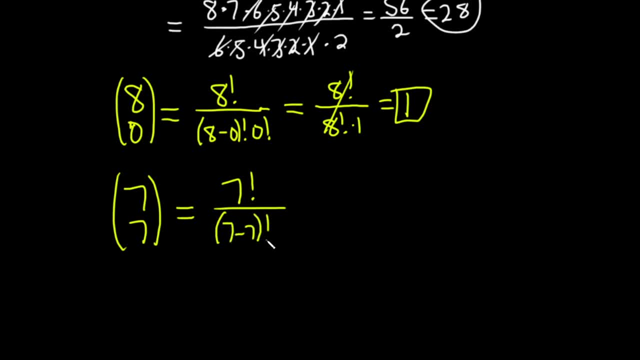 so this is your n and your r. so 7 minus 7 factorial and then r is again 7.. This is equal to 7 factorial over 7 minus 7 is 0, so we get 0 factorial, 7 factorial. 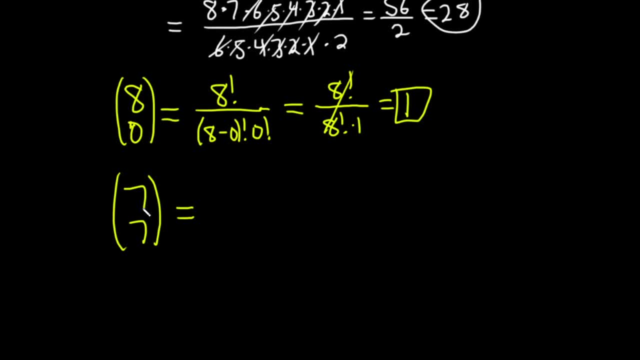 This one is saying: how many ways can you choose 7 objects from a group of 7?? There's one way: you choose all 7.. So the answer should be 1.. So it's 7 factorial over it's n minus r. 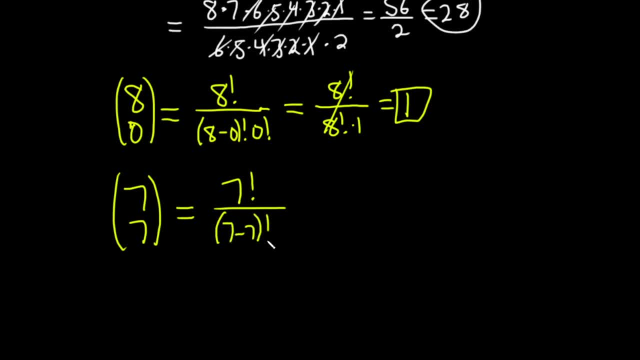 So this is your n and your r. So 7 minus 7 factorial and then r is again 7.. This is equal to 7 factorial over 7 minus 7 is 0.. So we get 0 factorial, 7 factorial. 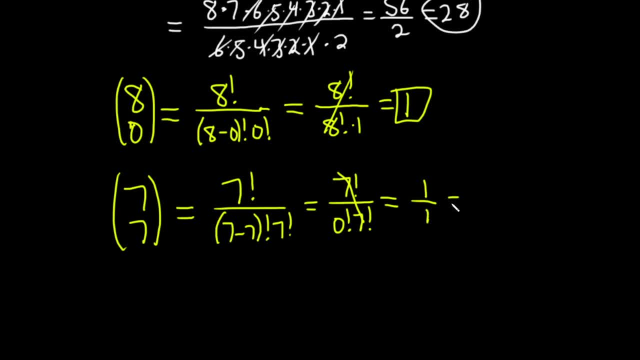 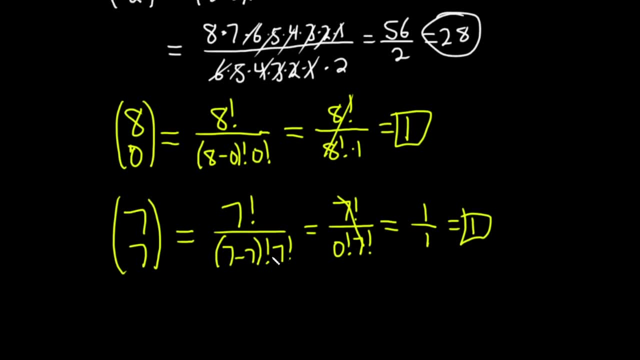 These cancel, So you get 1 over, and then 0 factorial is 1.. And so you just get 1 in this case as well. Pretty cool, right? Really not too bad. Let's do another one. How about? how about 7 factorial over 7 factorial? 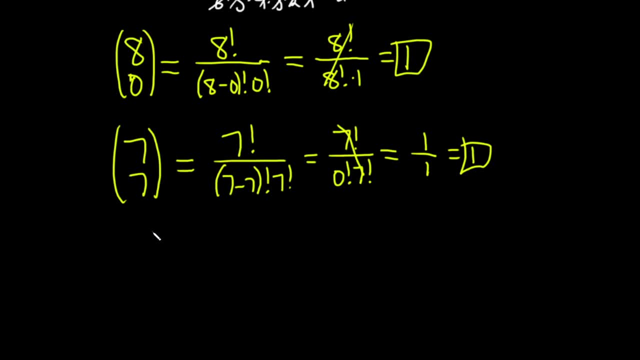 Let's just mix it up About 9, choose 5.. So again it's this one factorial. Then on the bottom it's n minus r, So 9 minus 5 factorial. Some people skip steps here. they'll put 4.. 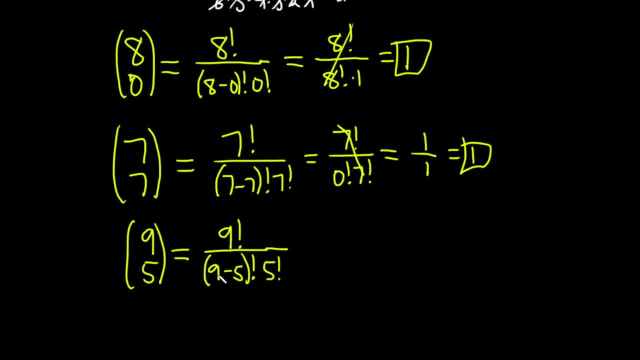 I don't like doing that, You know, I just don't like doing it. So it's n factorial n minus r r. This is n factorial. This is 9 factorial over. let's see: 9 minus 5 is 4 factorial. 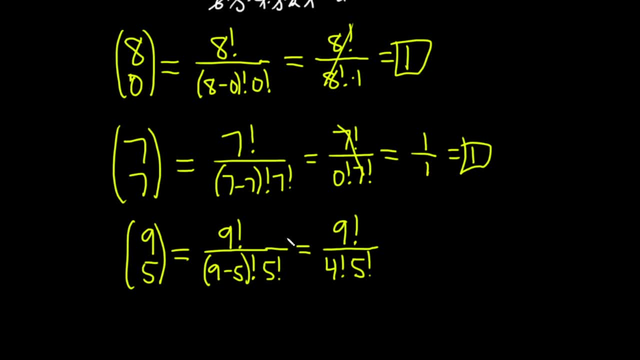 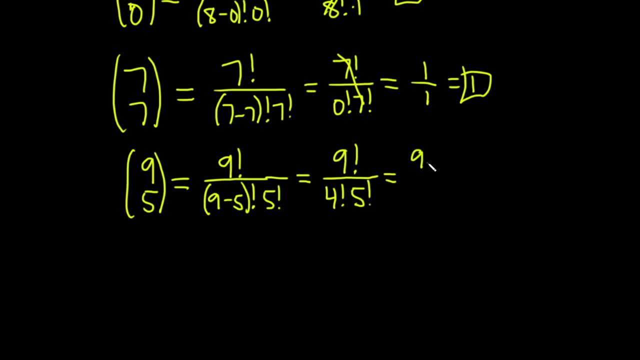 And then 5 factorial is 5 factorial. Okay, so this is equal to: let's see: so 9 factorial is 9 times 8 times 7 times 6 times 5, 4,, 3, 2, 1.. 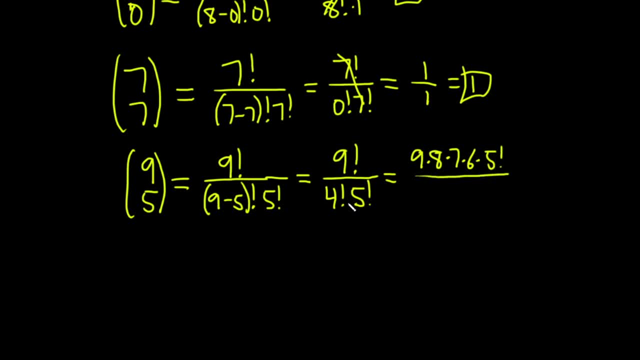 So 5 factorial over 4 factorial? Okay, Okay, Okay, 4 factorial is 24.. I haven't memorized. It's being cheap here Times And then 5 factorial Boom. So this is. I probably should have written out the 24.. 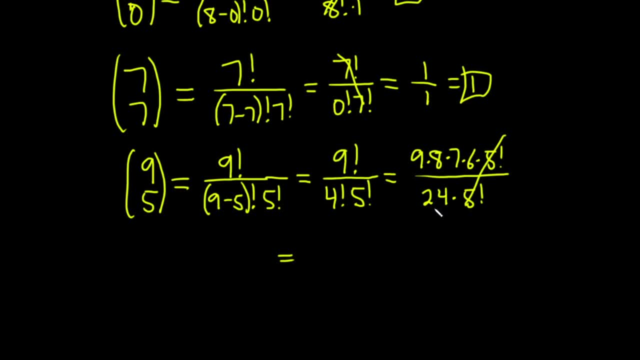 It might have made it easier to do. I'm kind of having some regrets there, but yeah, Maybe I will. 9 times 8 times 7 times 6.. This is 4 times 3 times 2 times 1.. 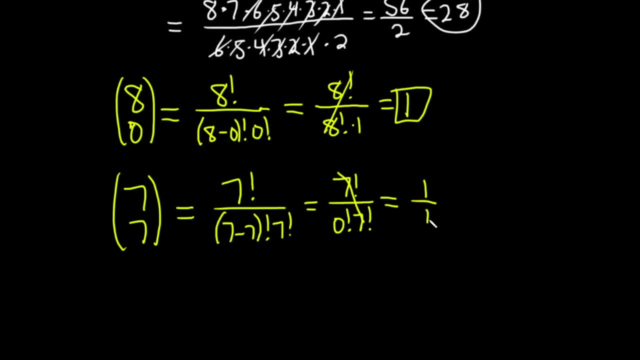 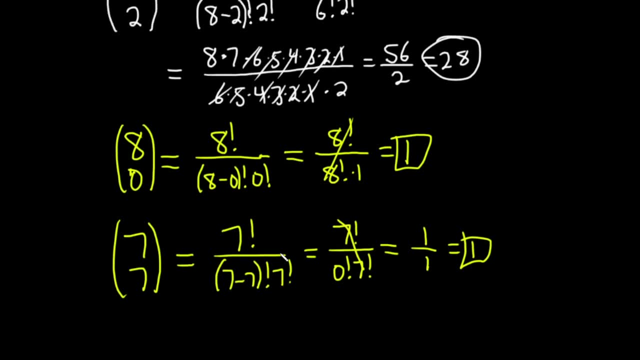 These cancel, so you get 1 over, and then 0 factorial is 1, and so you just get 1 in this case as well. Pretty cool, right? Really not too bad. Let's do another one. How about? 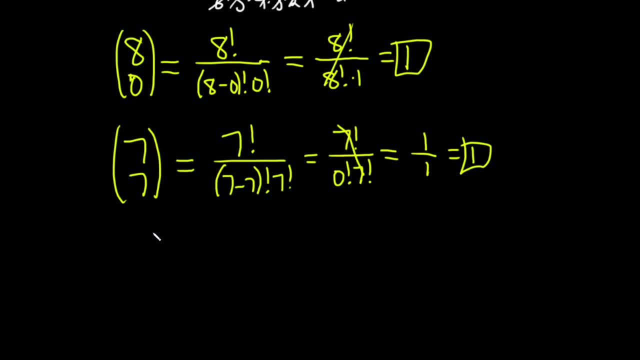 let's just mix it up about 9, choose 5.. So again it's this one factorial. then on the bottom it's n minus r, so 9 minus 5 factorial. Some people skip steps here. they'll put 4.. I don't like doing that. 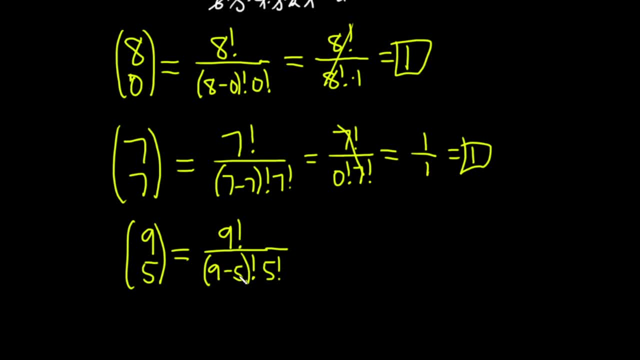 You know, I just don't like doing it. So it's n factorial n minus r r. This is 9 factorial over. let's see: 9 minus 5 is 4 factorial and then 5 factorial is 5 factorial. 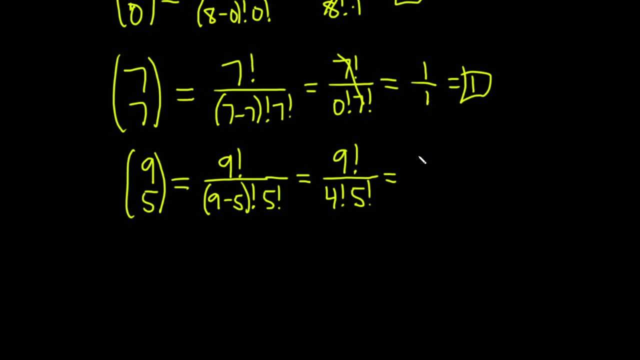 Okay, so this is equal to: let's see: so 9 factorial is 9 times 8 times 7 times 6 times 5.. 1, 2, 3, 4, 3, 2, 1, so 5 factorial over 4 factorial is 24, I haven't memorized. 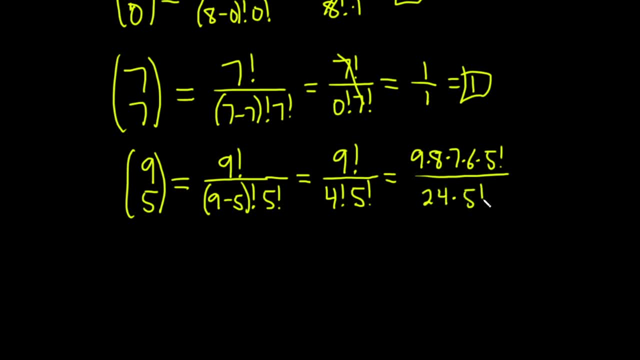 being cheap here times and then 5 factorial Boom. So this is. I probably should have written out the 24. It might have made it easier to do. I'm kind of having some regrets there, but yeah, maybe I will. 9 times, 8 times 7 times 6.. This is 4 times 3 times 7 times 6.. 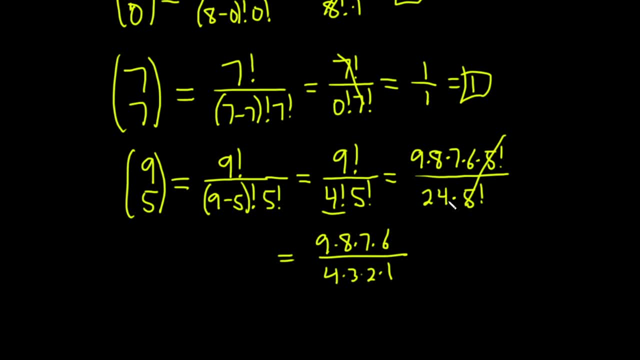 4 times 3 times 2 times 1.. That's 4 factorial. I don't know why I put 24, but skipping steps. So the 3 and the 2, they cancel with the 6, and the 4 goes into 8 twice, You see. 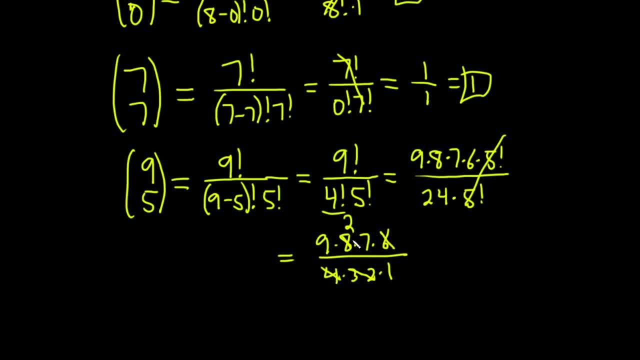 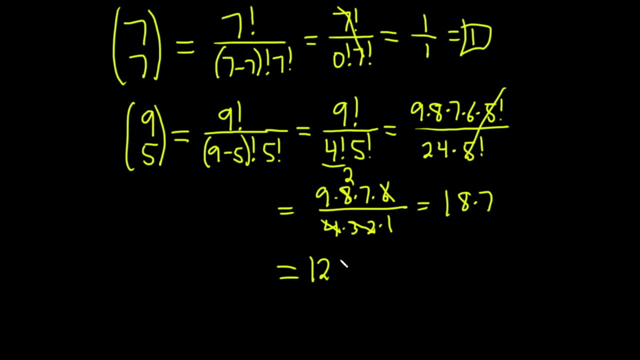 how much easier that is. 6 cancels with 6,, 4 goes into 8 two times, and so you get 18 times 7.. 18 times 7, which is 126,, I believe 126.. 126.. 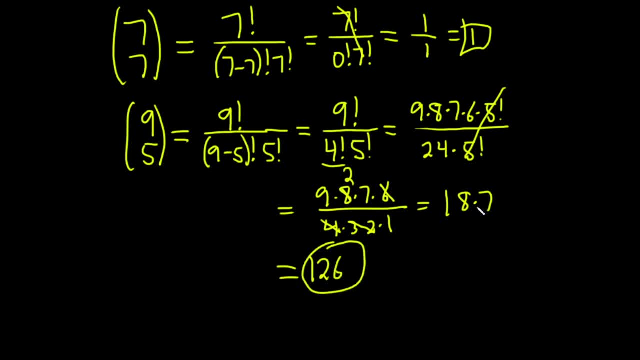